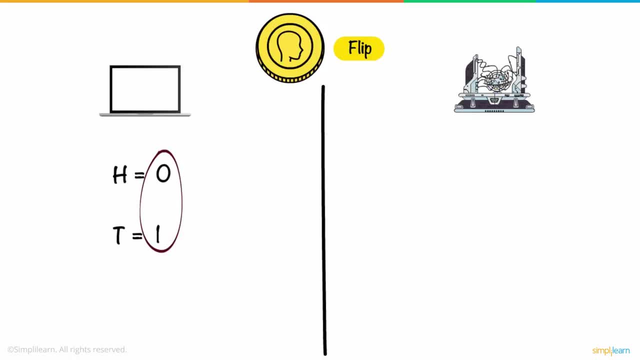 these two results, while the quantum computer, on the other hand, will also have these possibilities, including a possibility of a mixture of both heads and tails, like 0 and 1,, for example, with some portion of 0 and some portion of 1.. And due to this fluid possibility, it increases. 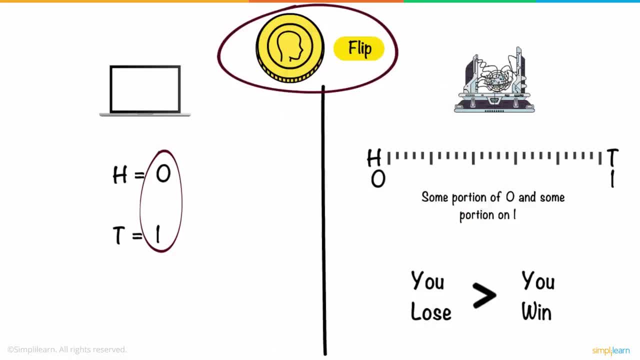 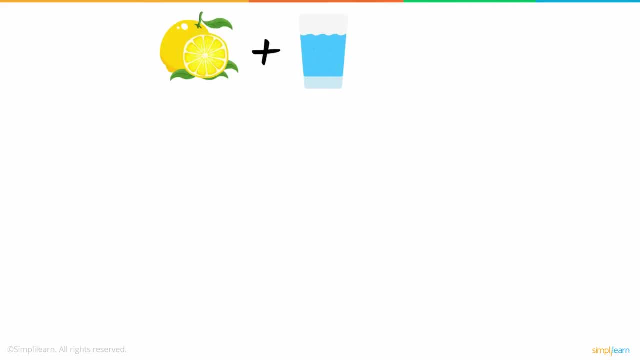 the chances of you losing the game, Because whether you choose to flip the coin or not, the outcome will still be there between both possibilities, Just like a mixture of lemon juice and water. even though the portion of lemon juice is very little in that mixture, you can't say that it is not there. This property of superposition and 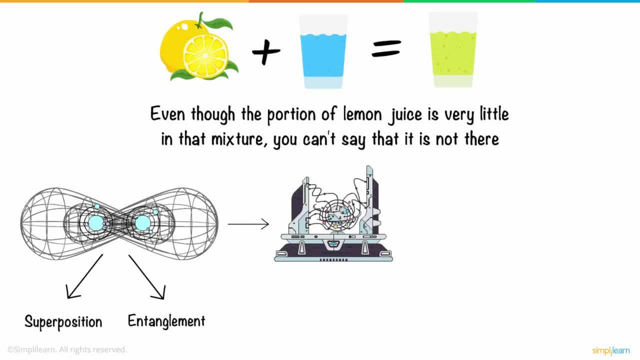 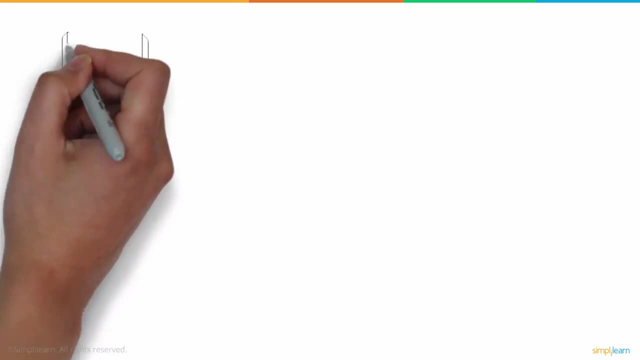 entanglement of quantum physics empowers quantum computers to handle operations at speeds that are orders of magnitude faster than traditional computers, while using a fraction of the energy. Upon understanding this, Dave was mesmerized by the concept of quantum computers. Quantum computers aims to revolutionize more future quantum technologies And, just like 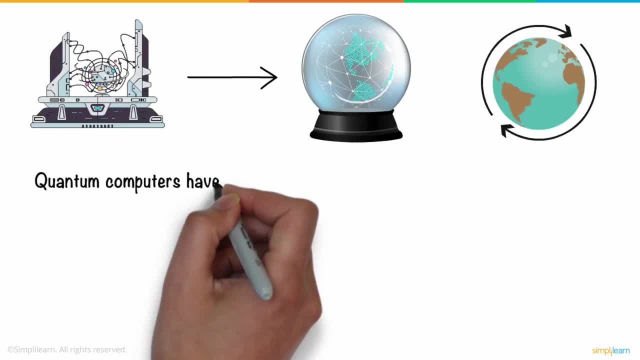 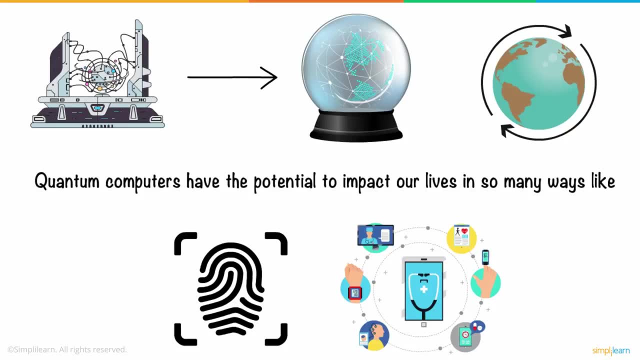 other transformations, quantum computers will also revolutionize the future of quantum technology. And just like other transformations, quantum computers will revolutionize the future of quantum technology. And just like other transformations around the world, quantum computers have the potential to impact our lives in so many ways, like our security needs, healthcare needs, etc. 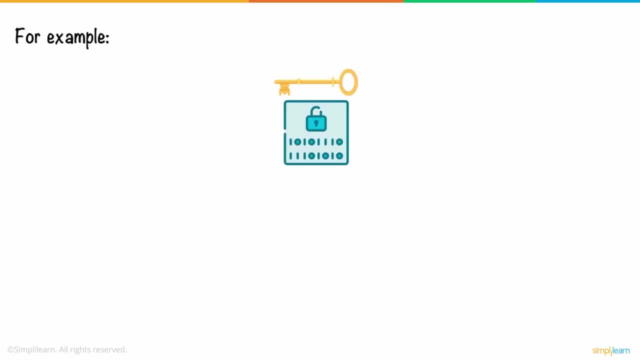 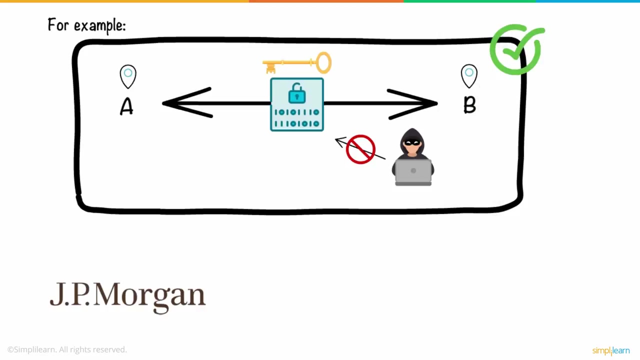 For example, it can be used to create private keys for encrypting messages from one location to another. It can be difficult for people with ulterior motives to copy the key of quantum uncertainty. This type of unique and unbreakable encryption is already tested by banks and companies like JP Morgan, Wells Fargo, Barclays. 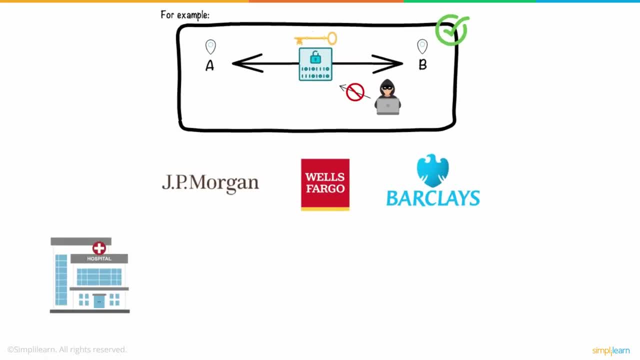 etc. It can be used in the medicinal world, as it will be easier for quantum computers to study each property of atoms and molecules, as it works on a similar concept. So here is a question for you: What makes quantum computers different from supercomputers? 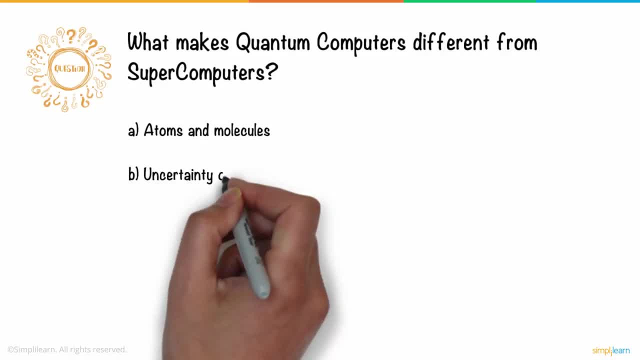 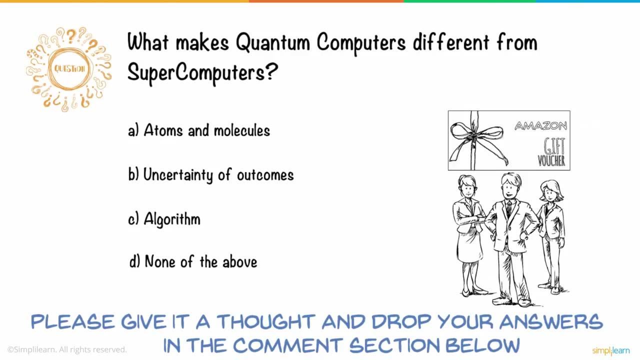 A- Atoms and molecules. B- Uncertainty of outcomes. C- Algorithm D- None of the above. Please give it a thought and drop your answers in the comment section below. Three lucky winners will receive Amazon gift vouchers. Due to its benefits, currently it is connected to over 17 billion devices globally.